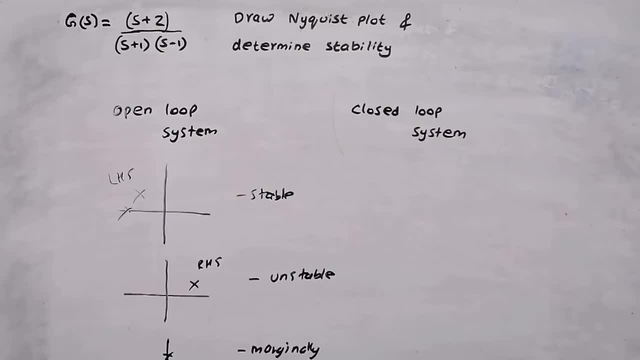 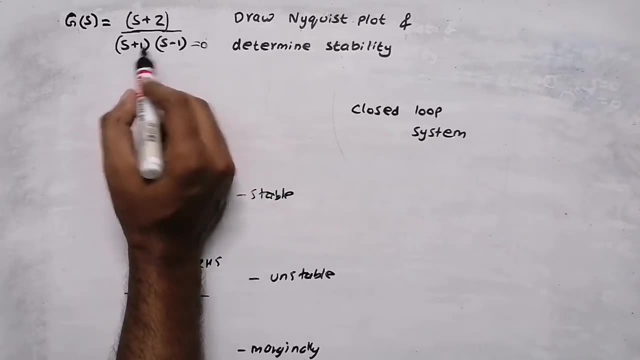 are the cases in open loop system. So in this question to find poles, what we will do, We will equate denominator equal to zero. When we equate denominator equal to zero, we will get either s plus 1 equal to zero or we will get s minus. 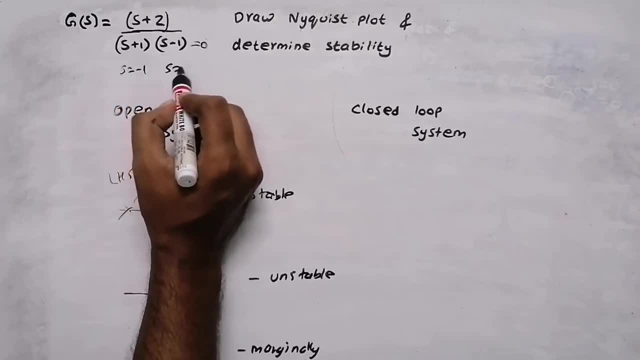 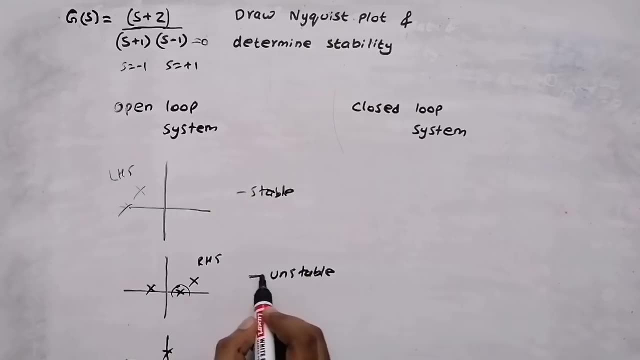 1 equal to zero. From this we will get s equal to minus 1.. From this we will get s equal to plus 1.. So minus 1 and plus 1.. So there is a pole on the right hand side. Therefore, this system will be unstable. Open loop system will be unstable, But we 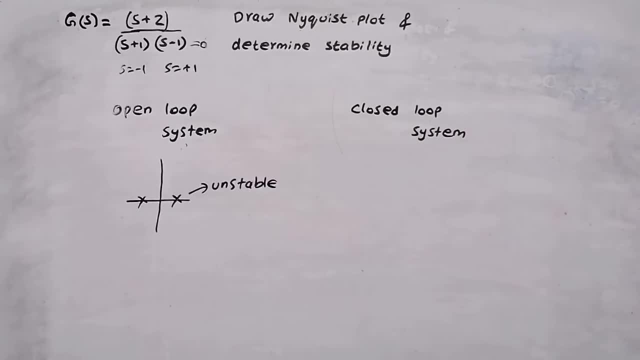 need to find the stability of closed loop system. So in this question the open loop system is unstable, but we need to find the stability of closed loop system. As we know, transfer function of a closed loop system is g divided by 1 plus gh. 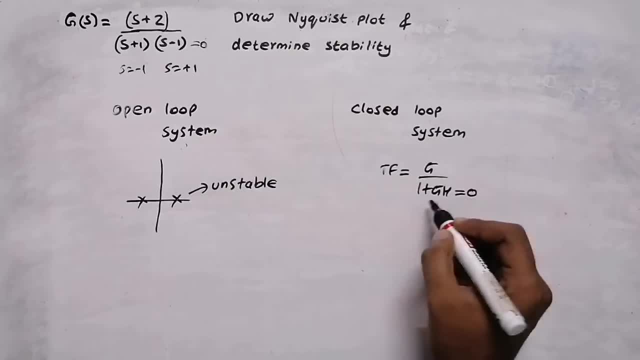 For getting poles. what we will do? We will equate denominator equal to zero. From this we will get 1 plus gh equal to zero. That means gh equal to minus 1.. So for determining the stability of closed loop system, we will draw a plot in gh plane. 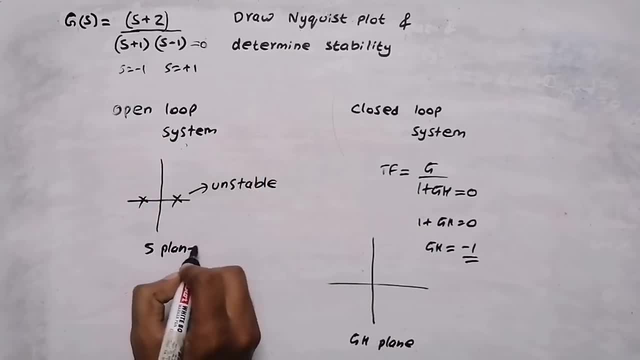 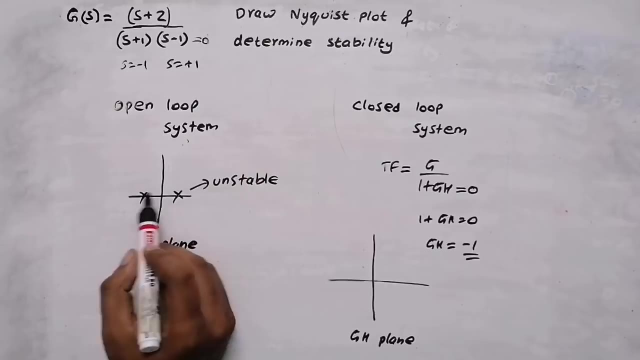 For open loop system, we draw a plot on s plane and located the poles. If poles are on the average axis system will be unstable. For closed loop system, for determining stability, we will draw plot on gh plane. Okay, in gh plane. Here we are determining with respect to the origin, If it is on the left hand side. 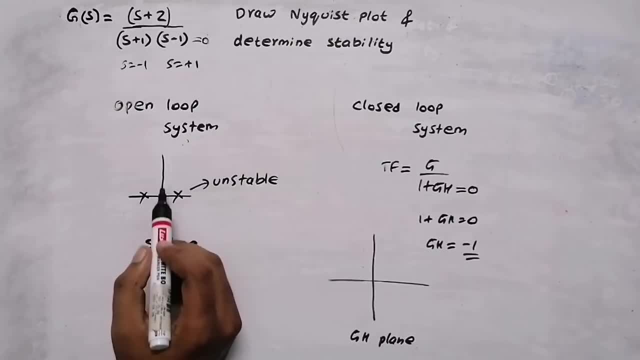 system is stable. If it is on the right hand side, system is unstable. If it is on the imaginary axis, system margin is stable. Here we are going to determine with respect to minus 1.. With respect to this point, we are going to. 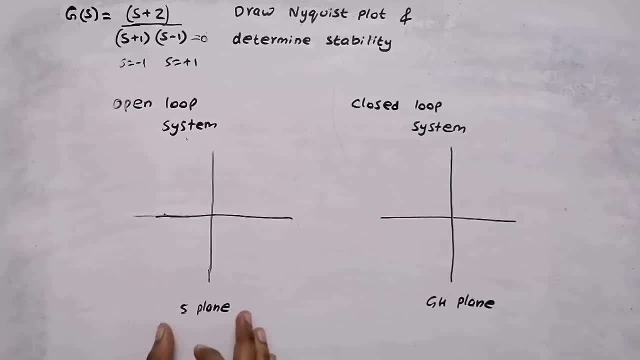 determine the stability. So by using S plane we are going to plot gh plane And the process is called as mapping. We studied it in engineering mathematics: complex analysis From Z plane to W plane mapping. It is a process. so by using s plane, we want to find gh plane. for that purpose we are going to use the 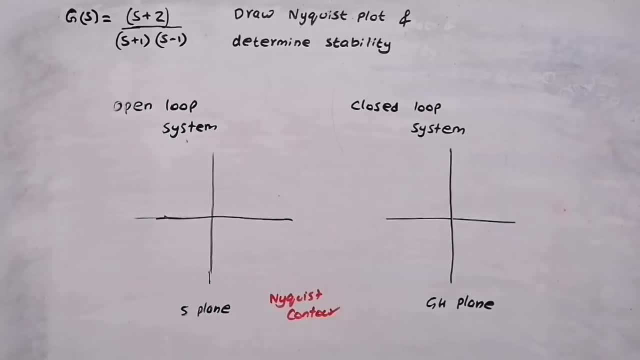 help of nyquist condor. okay, as we know, if a pole is there on the right hand side, system will be unstable, so we are going to take the entire right hand side. that means starting from the origin. this is real axis and this is j omega axis. starting from origin means when omega equal to 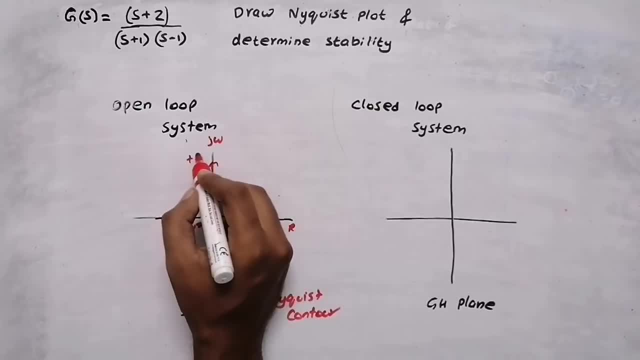 zero, then up to infinity, up to positive infinity. that means up to omega equal to positive infinity. we are taking our first region. i'm going to name it as c1. c1 is my first region, that is, from omega equal to zero to omega equal to positive infinity. then i'm going to take the entire right hand side. 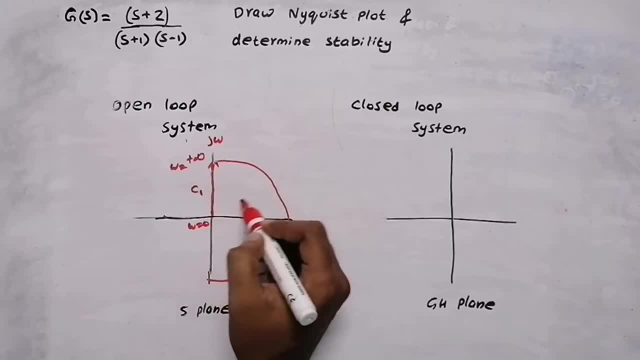 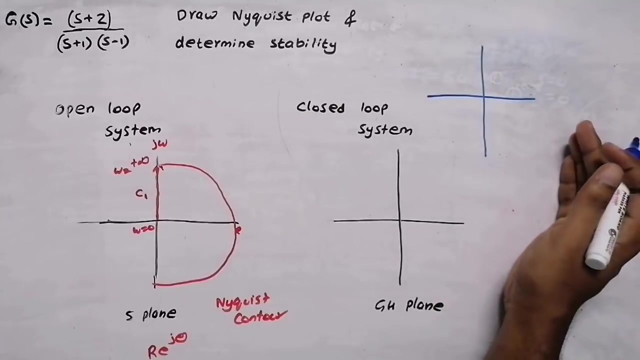 plane, entire right half. okay, that means the radius of this. this is circle. okay, so in polar plot the equation of circle is r, e raised to j, theta, where r is the magnitude or radius of the circle and theta is the angle. okay, as we know in polar plot. why i'm saying about polar plot is that nyquist plot. 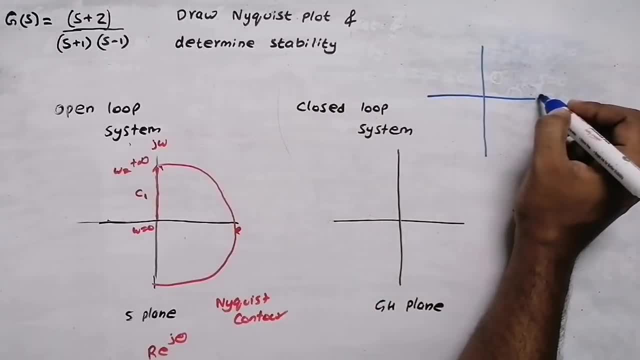 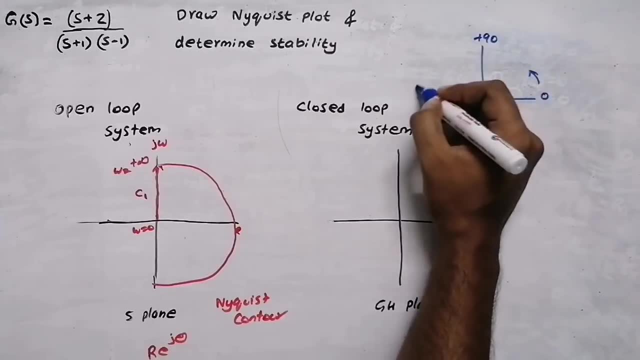 is an extension of polar plot. okay, so in polar plot, the angles are taken positive in anti-clockwise direction. if it is in anti-clockwise direction, angles are positive. this is zero, this will be plus 90, this will be plus 180, this will be plus 270. and in clockwise direction angles are taken. 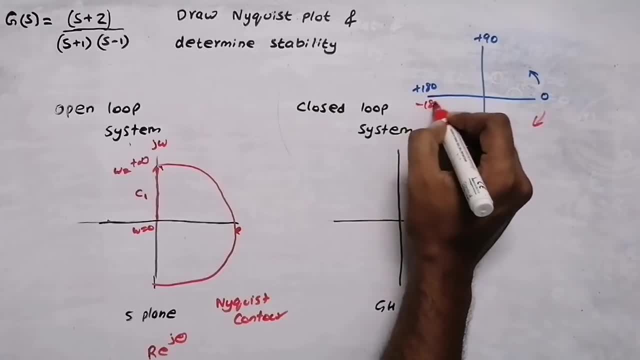 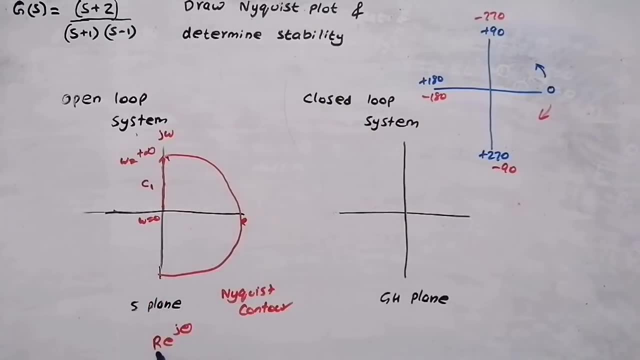 negative. if this is zero, this will be minus 90 minus 180 minus 270. so angles are taken negative, in anti-clockwise direction. so for this circle the radius r will be infinity, because we will cover the entire right half plane. so the radius of the circle will be up to infinity. what about theta? theta is starting from here, that is. 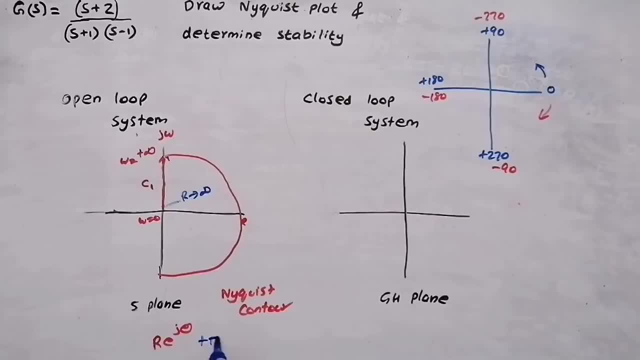 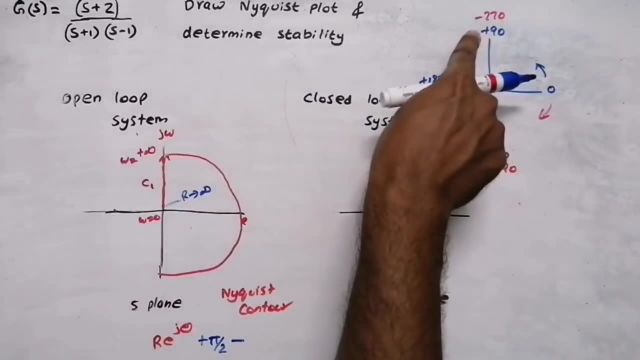 plus 90, that will be plus 90. i can write it as pi by 2 in radian. okay, pi by 2 to up to how much? up to this point, that is minus 90, from plus 90 to minus 90. so plus pi by 2 to minus pi by 2, that is. 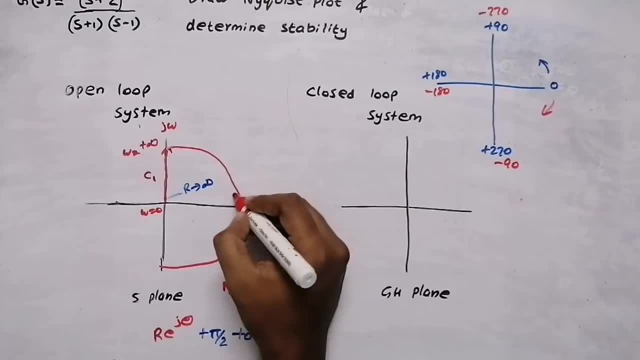 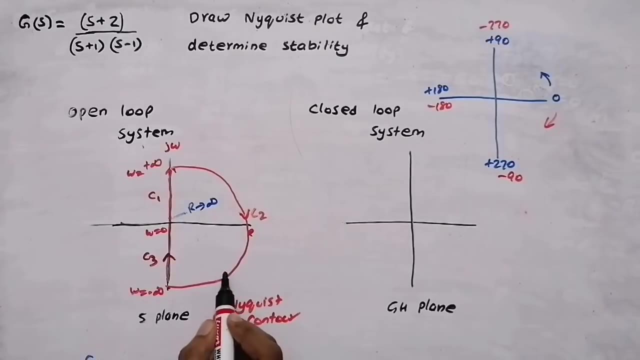 angle theta. i'm going to name that region as c2. now, after reaching here, then this is our j omega axis. so from omega equal to minus infinity to omega equal to 0, that is my third region. i'm going to name it as c3. this is the nyquist contour of. 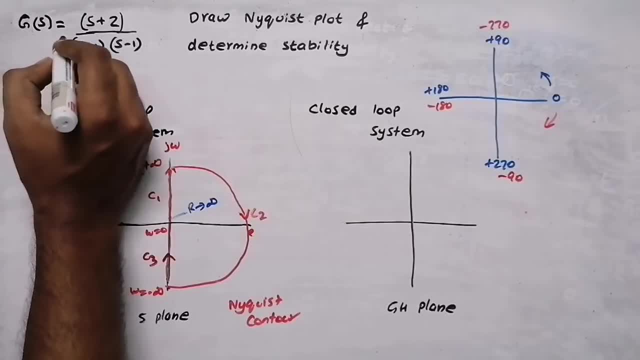 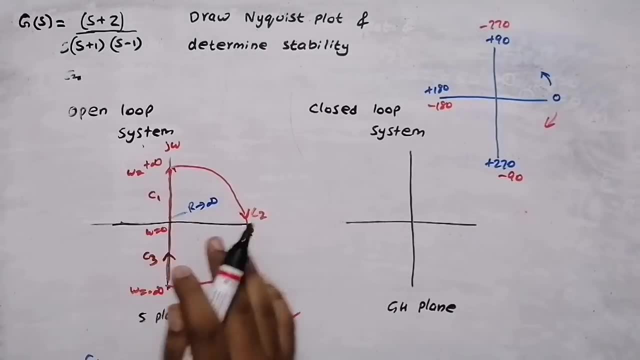 this system. if suppose think that there is a pole here, okay, then we will get s equal to zero. that means a pole will be there at the origin. at that time there will be slight difference in the nyquist contour i will discuss in the next video. i will do a problem with when there is a pole at origin. 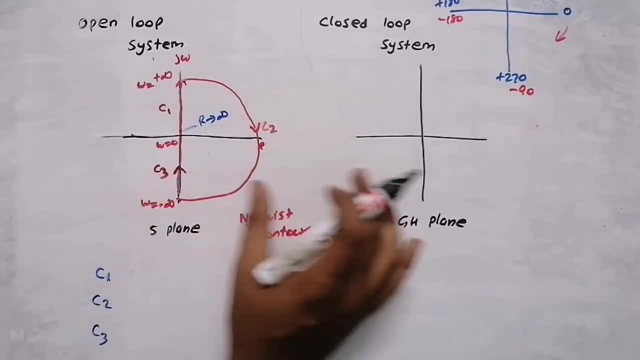 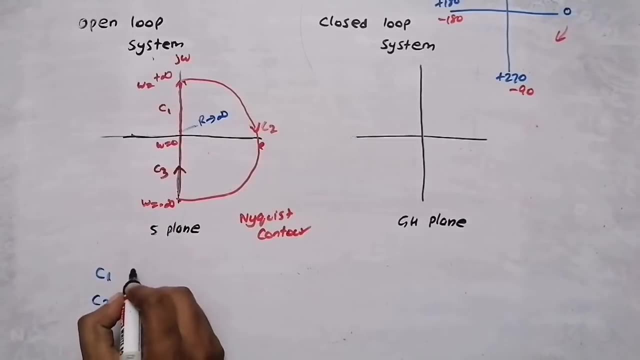 so this is my nyquist contour. using this nyquist contour, i need to plot gh plane. okay, so this nyquist contour consists of three regions: c1, c2 and c3. c1 is the region when omega equal to zero, to omega equal to infinity. at that time, using this s plane, i need to plot gh. so wherever there is s, i need to. 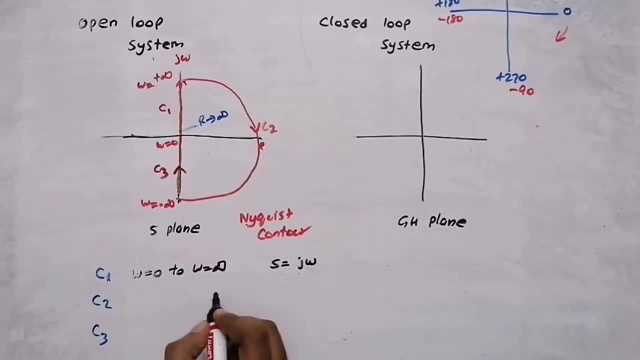 replace it with j omega. okay, then the next plane. next point is the entire right hand side. that means r turns to infinity. at that time, instead of s, i need to substitute r, e raised to j theta. here r tends to infinity, so limit r tends to infinity. r e raised to j theta. instead of s i need to substitute. 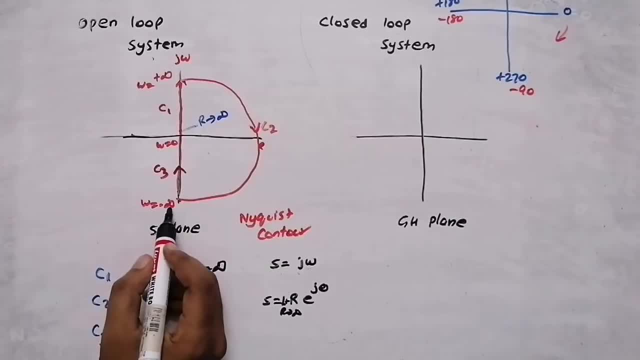 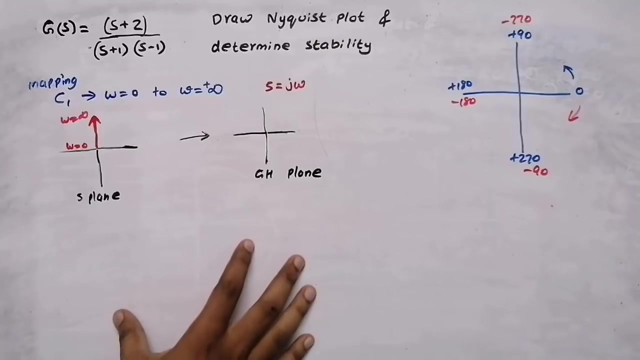 this: c3 is the region when omega is minus infinity to omega, equal to zero. so omega is minus infinity to omega, equal to zero. at that time, instead of s i need to substitute j, omega, but this time my omega varies from minus infinity to zero. so now i am going to map my first region, that is, c1. 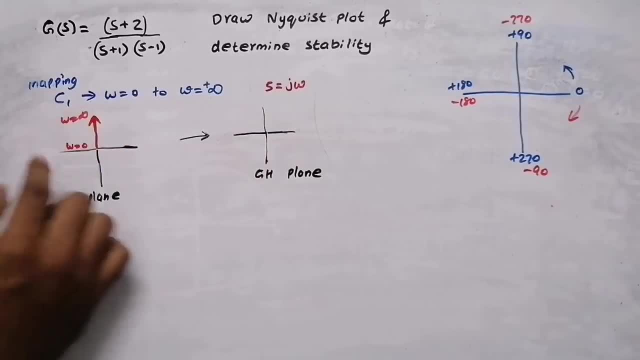 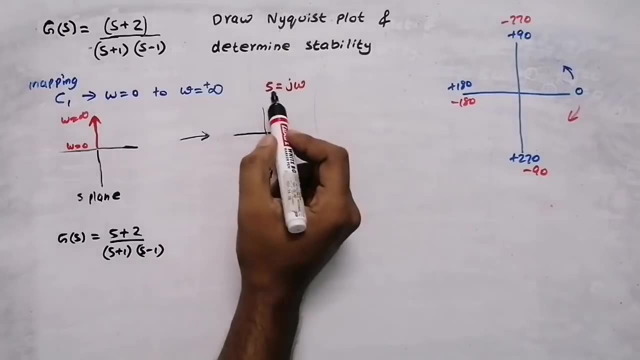 where omega varies from zero to positive infinity. this is in s plane. we are going to find what will plot in gh plane. so in this case, this is our question g of s. so wherever there is s, it should be replaced by j omega. but before doing that we need to check whether our question is in standard. 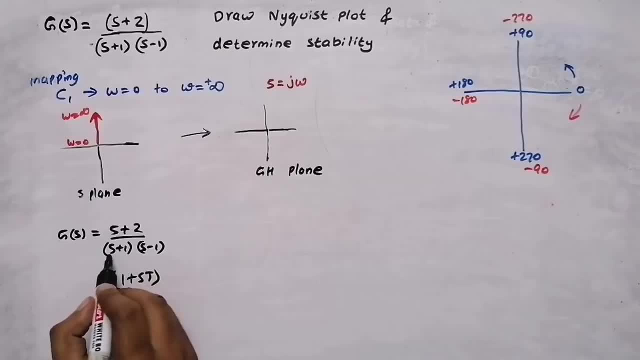 form, that is one plus st format. here it is one plus s, here also minus one plus s, but here it is two pluses. so instead of two we need to make it as one. so what we will do, we will take this two outside. so it will become: i am taking two outside, then i am going to write it as one plus s s by two. 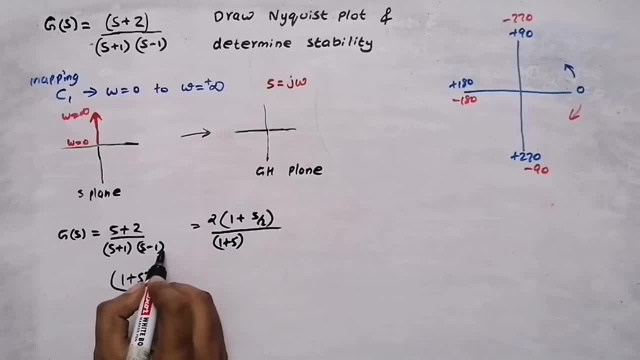 divided by- here it is of the form one plus s. then here i am writing in the reverse: okay, so minus one, then plus s. so this will be my standard form. so if i am writing two, one plus s by two, one by two, it will be point five. so point five s divided by one plus s, then minus one plus s. 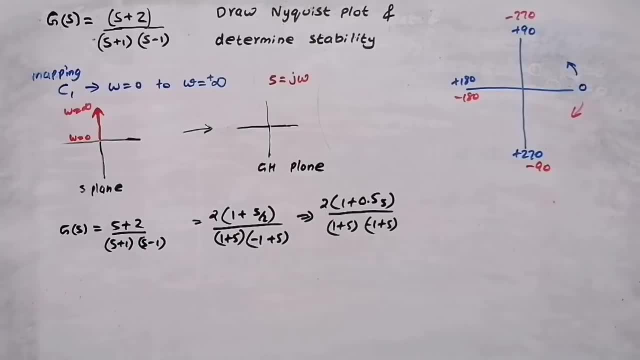 now my g of s is in the standard form. okay, now i am going to replace: instead of s, i am going to write j omega. so wherever there is s, i need to replace it with j omega. so wherever there is s, i replace it with j omega. so this is g of s, this is my g of j omega. 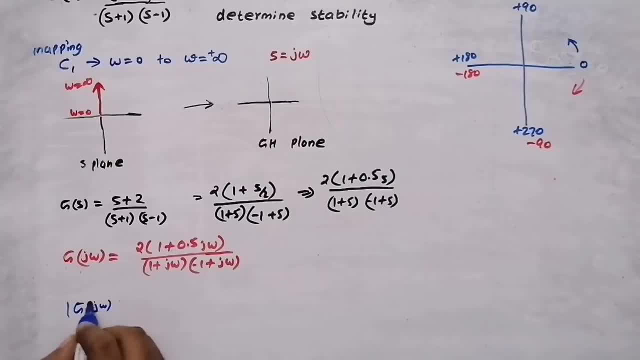 now i need to find the magnitude g of j omega's magnitude and face angle angle of g of j omega. so first of all i am going to find the magnitude. what will my magnitude? two, and here it is for the format a plus b. so magnitude: it will be root of a square plus b. square root of a. a is one one. 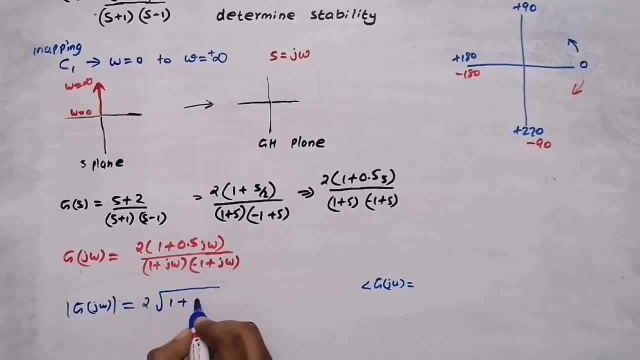 square, it will be one itself plus b square. it is point five omega. so point five omega square. divided by so denominator, it is one plus j omega, so a plus b format, a plus ib format, so the magnitude of a square plus b square ab, you don't want to take this item. the magnitude will be root of a square. 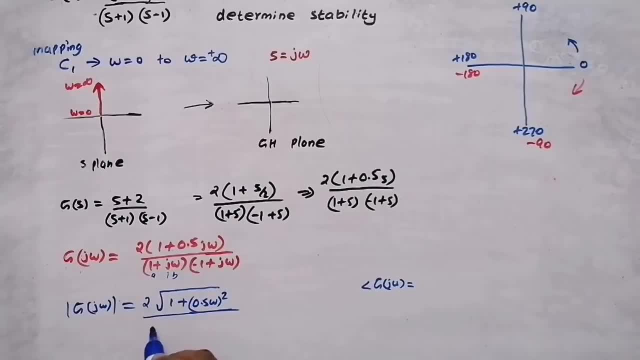 plus b square. so root of a square it is one, one square it is one. then b squared it will be omega square. so one plus omega square, and here it will be minus one square. it will be one plus omega square. so this will be my magnitude now. angle of g of j, omega, taking the first exam. 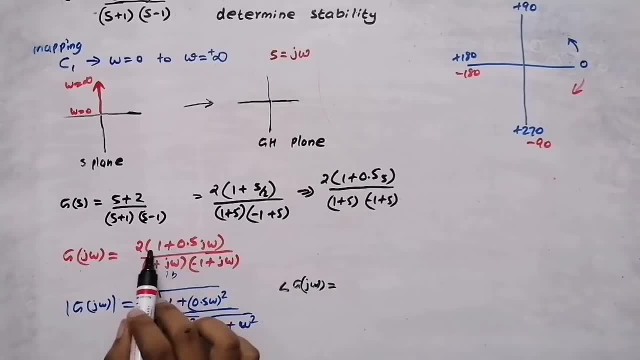 here it is in the numerator. so angle will be positive. a plus b format. therefore tan inverse b by a, b, it is positive right. so this is a positive foi in sEC. 0.5 omega, 0.5 omega divided by 8 is 1.. So 0.5 omega by 1, it will be 0.5 omega itself. 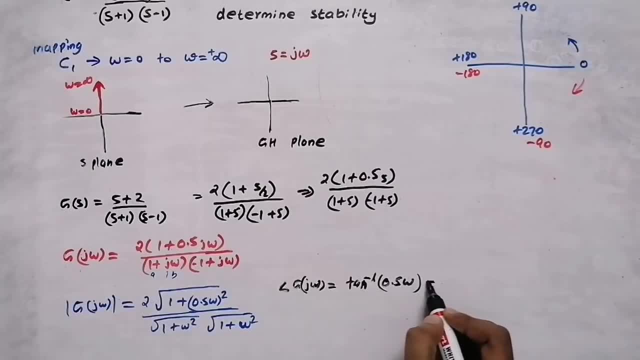 Now in denominator denominator, then it will be negative sign Here also the format A plus B format, So tan inverse: B by A, B it is omega, A it is 1.. So omega by 1,. 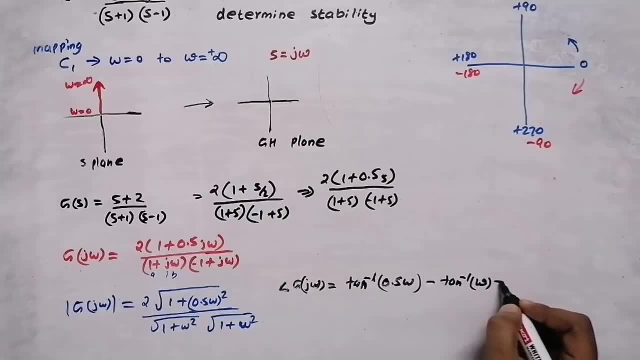 it will be omega itself. Then this term is also in the denominator, So negative sign. Then tan inverse B by A, B it is omega, Then A it is minus 1.. So omega by minus 1,. 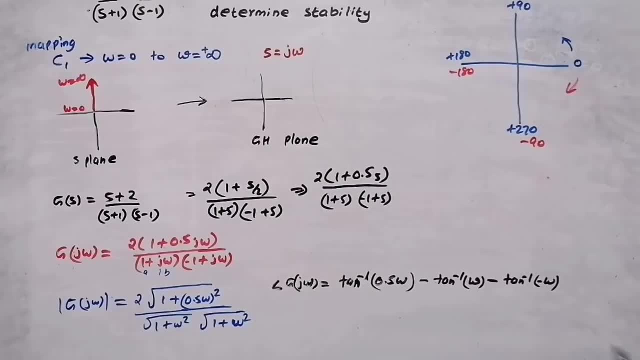 it will be minus omega. Now, instead of this tan inverse minus omega, I am going to rewrite it as 180 minus tan inverse omega. Instead of minus omega, I replace it with tan omega. So instead of this term, I am going to write this term. So my angle will be: tan inverse 0.5 omega minus. 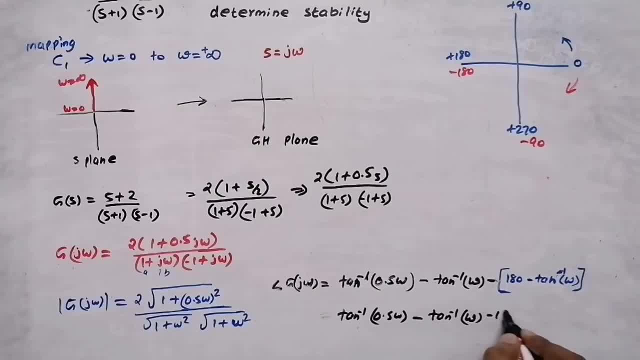 tan inverse omega, then minus 180,, minus and minus, it will become plus, plus tan inverse omega. Now this minus tan inverse and plus tan inverse omega will cancel out. Then the remaining term. it is minus 180,. 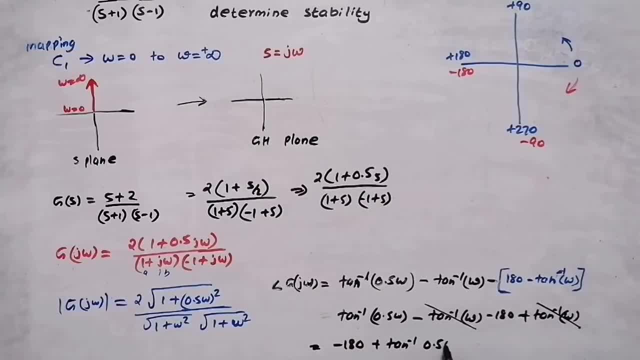 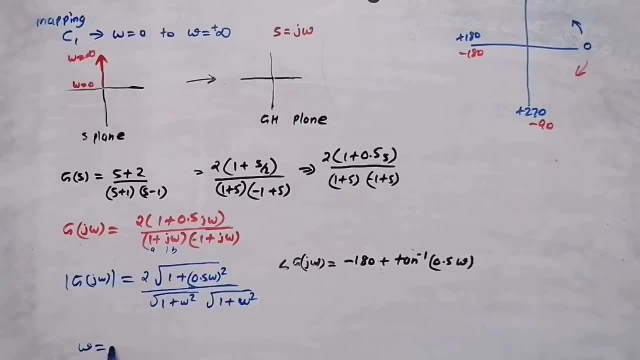 then plus tan, inverse, 0.5 omega. So this will be my phase angle. Now our omega is varied from 0 to infinity. So first of all, I am going to take omega equal to 0. I am going to find the. 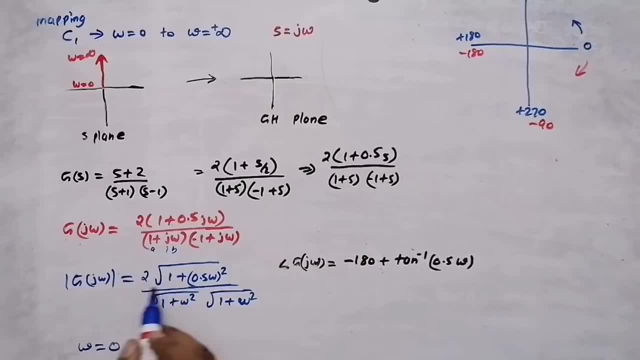 magnitude and phase angle when omega equal to 0. So magnitude it will be. when I am substituting 0 here, it will be 1 plus 0.. Anything added to 1 plus 0, it will be 1 itself. So 2 into root 1,. 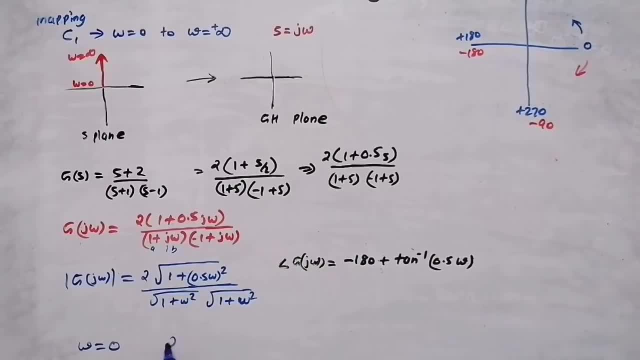 then here also 1.. So the magnitude that I am going to get will be 2.. Now phase angle: when I substitute 0, omega equal to 0, when I substitute 0 here, it will become minus 180 plus tan inverse 0. What is tan inverse 0? Tan 0 is 0. So tan inverse 0 will be 0 itself. 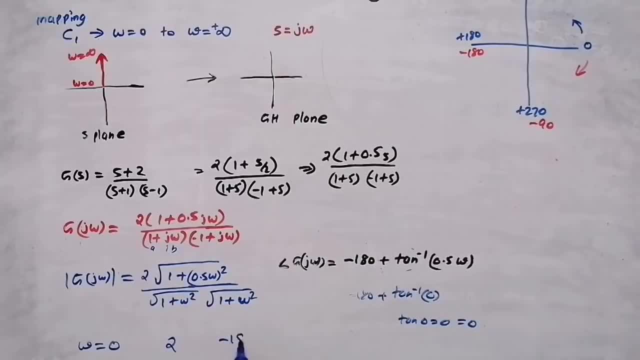 So this term it will be 0. Then the angle I am going to get is minus 180.. So magnitude it will be 2, and the angle it will be minus 180.. Now, when I substitute omega equal to 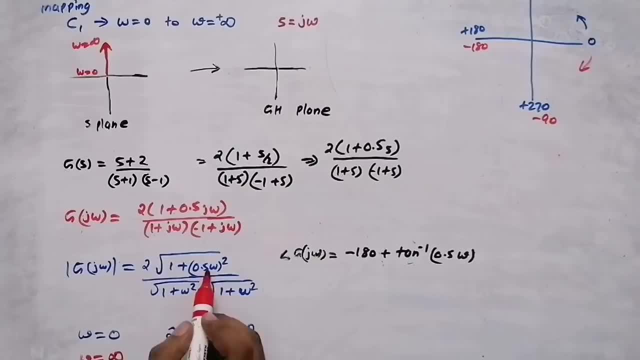 infinity, So omega equal to infinity. in this equation For finding magnitude I am going to substitute omega equal to infinity, So 1 plus infinity. anything added to infinity, it will be infinity. Now here infinity is coming in the denominator side, So 2 divided. 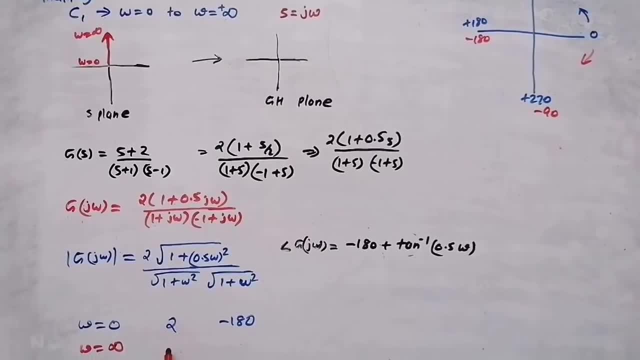 by infinity. anything divided by infinity, it will be 0.. Okay, anything divided by infinity: 1 by infinity, it will be 0. So 2 by infinity will be also equal to 0. So magnitude will be 0.. Now for finding phase angle. substitute omega, equal to infinity, in this equation. 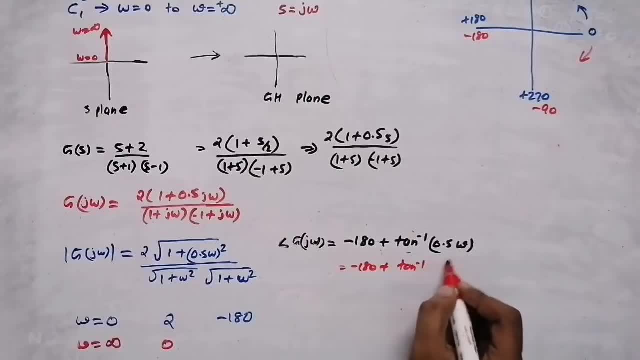 it will become minus 180 plus tan inverse 0.5 into infinity. It will become tan inverse infinity. What is tan inverse infinity? Tan 90 is infinity, So tan inverse infinity. it will be 90 degree, So minus 180 plus 90, it will be minus 90 degree, So the angle it is going to be. 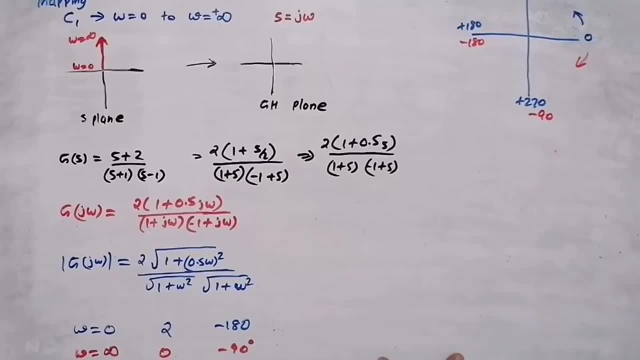 minus 90 degree. So region 1, from omega 0 to omega infinity. I need to replace s with j omega. So this is my question: g of s, I replaced it with g of j omega. So wherever there is s, I replaced it with omega. Then I found the magnitude, Then I found the phase. 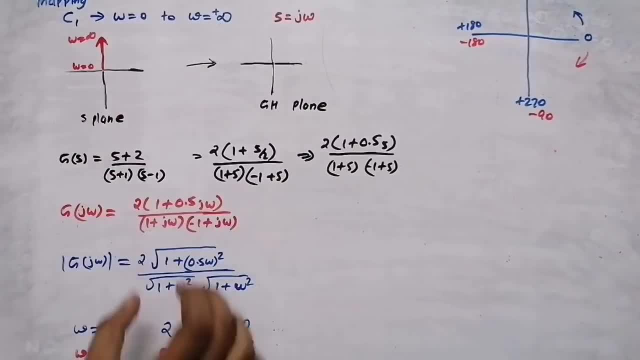 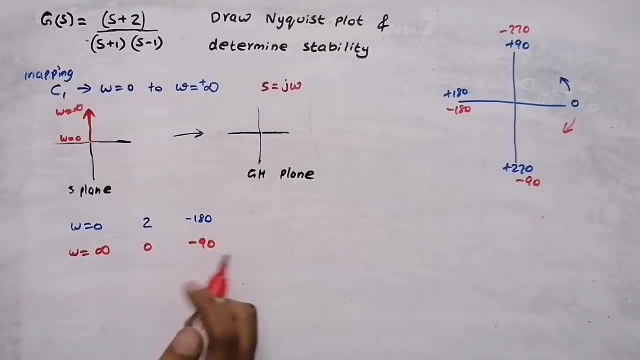 angle. Then for omega equal to 0,, I found the magnitude and phase angle. Then omega equal to infinity: also I found the magnitude and phase angle. Now I am going to plot these points in this graph. So omega equal to 0,, instead of this point in gh plane, it will be 2.. So if this is, 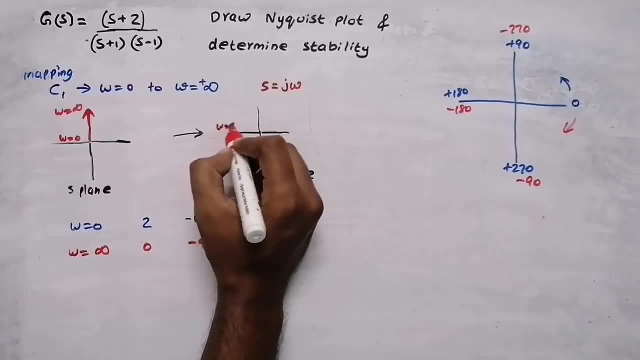 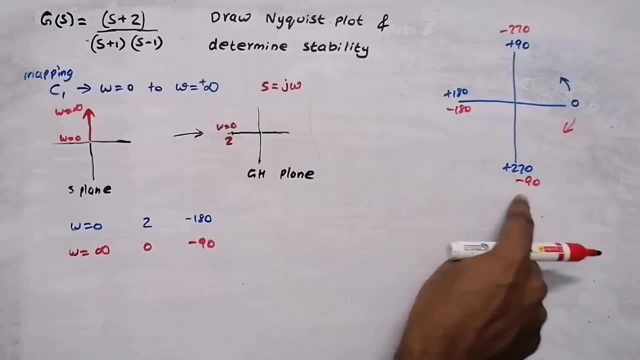 1, this will be 2.. So here, when omega equal to 0, it will be here 2, okay, magnitude 2.. Then phase angle: it is minus 180.. So 0, minus 90, minus 180.. So, starting from, 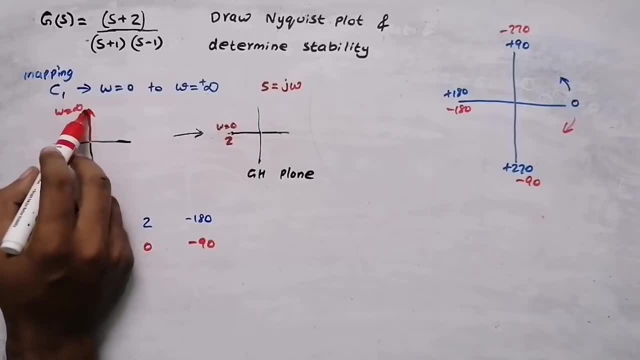 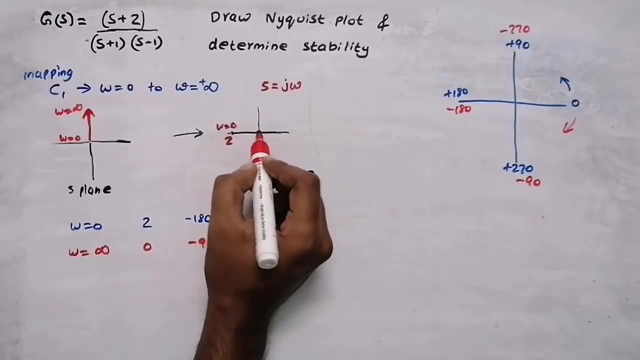 this point. okay, Now when omega equal to infinity, here it is, in s plane, it is here. So, mapping in gh plane, we will get 0 as the magnitude. That will be origin, Then angle, angle it is minus 90.. So minus 90 is this: 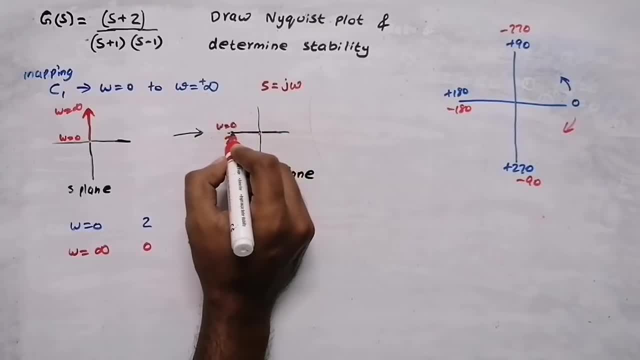 So it is going to end in this quadrant. okay, So, starting from here, starting from omega equal to 0 to infinity, the region is like this: Here, starting from 0 to infinity, the graph will be like this. The direction will be like this: In s plane, the region, 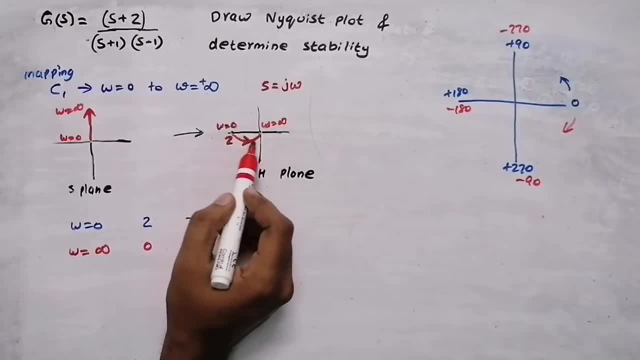 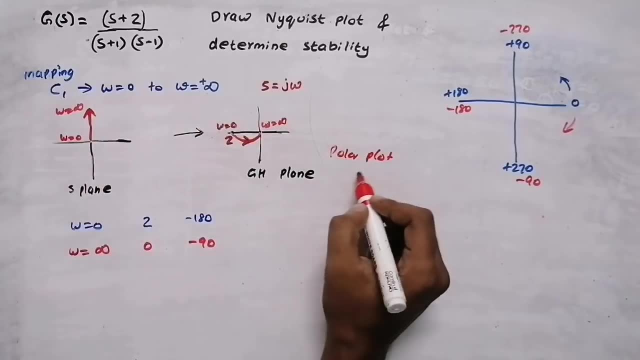 will be like this: In gh plane, the corresponding mapped region will be like this: This is our polar plot. okay, Plotting region from omega equal to 0 to infinity. In polar plot we will vary omega from 0 to infinity. 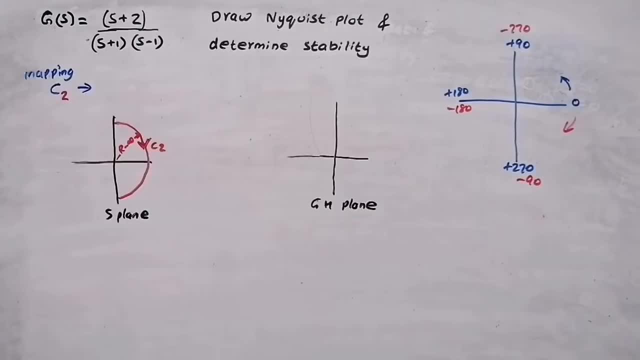 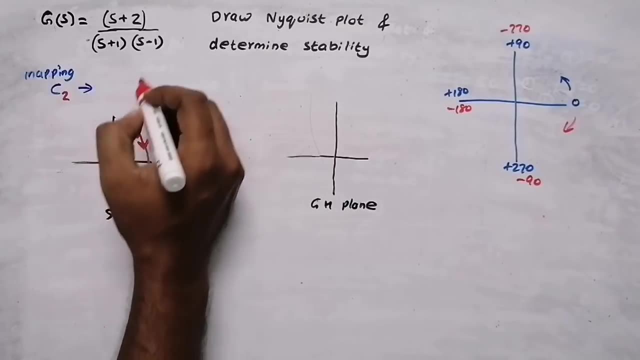 So this is the first region. Now we need to find the second region. Now I am going to map my second region, That is, this region In s plane. it is the entire right-hand side plane with radius infinity. So instead of s here, it is in s plane. I need to replace. 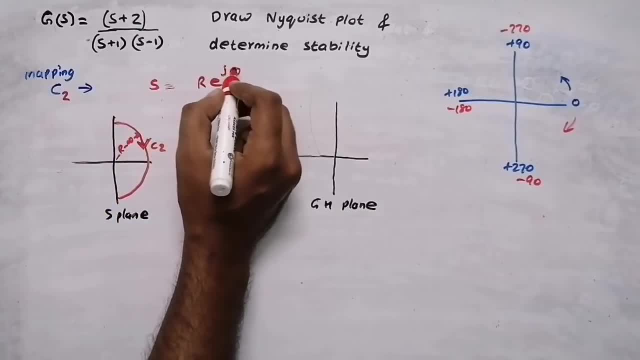 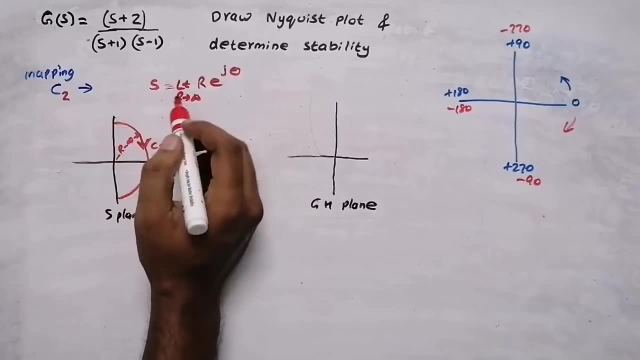 it with r, e raised to j theta. okay, My r. the radius is infinity, So I am going to write limit: r tends to infinity, Radius is turning to infinity, So instead of s, I need to replace this term. So this is my g of s in standard form. Wherever there is s, I 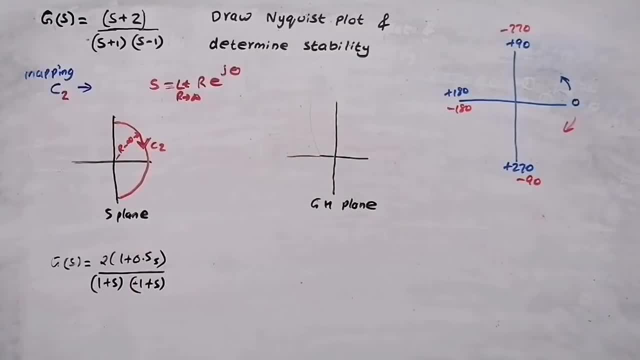 need to replace it with this term. okay, Before replacing, you need to reduce this g of s. I will tell you here: s is r, e raised to j theta and r is turning to infinity, So s will be new, s will be. r tends to infinity, So instead of r we can write infinity e. 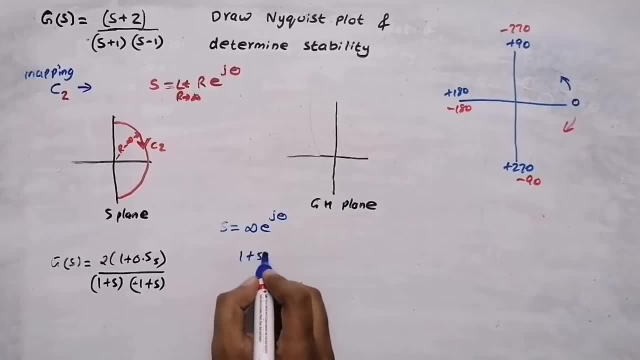 raised to j theta. okay. So 1 plus st- Instead of s, we are going to write this term- The magnitude will be infinity. So instead of s, the magnitude will be infinity. So anything added to infinity, we will get infinity itself. So instead of 1 plus st, we can write st. 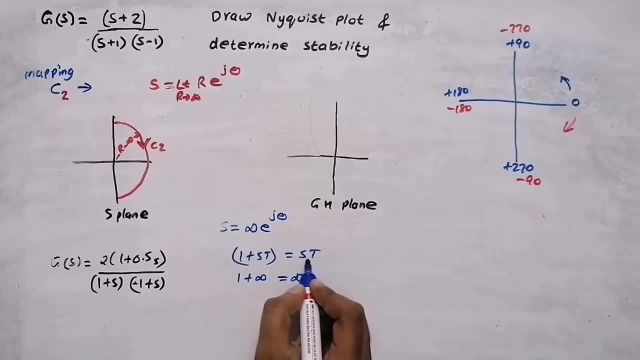 1 plus infinity. So 1 plus st will be st. So we can remove the 1s from all these terms. So by removing 1, we will get 2 into instead of 1 plus we can remove this 1.. Then the remaining. 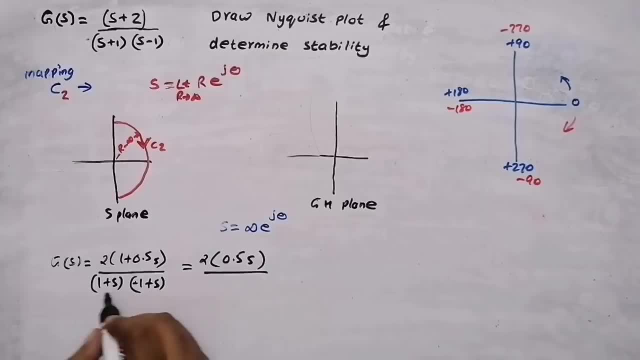 time it will be 0.5 s divided by removing this 1.. Here, removing this minus 1, it will get s Like this: This s and s will get cancelled, Then 2 into 0.5.. 0.5, it is 1 by 2.. So 2. 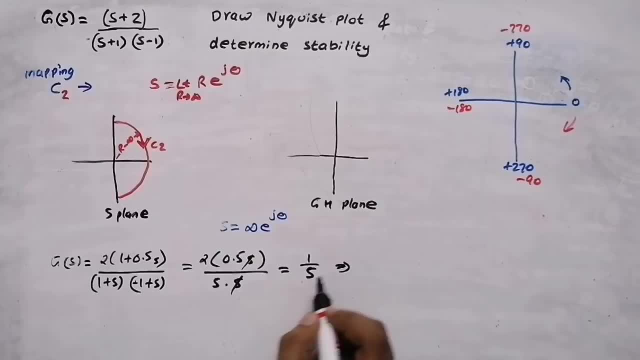 and 2 will get cancelled. We will get 1 by s. Now, instead of this s, we are going to replace it with infinity e raised to j theta, So it will become 1 by infinity e raised to j theta. 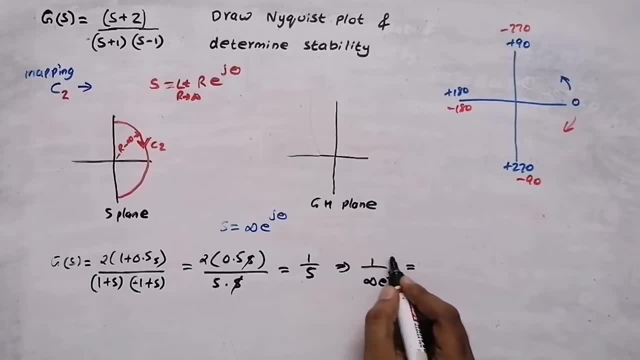 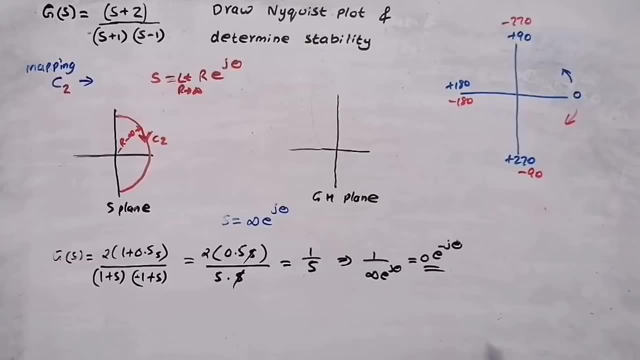 Now I am going to take this e raised to j theta in the numerator side, Then it will become e raised to minus j theta And you know, 1 by infinity it will be 0. So the magnitude will be 0 and theta is the angle. What is theta? Okay, Here theta is varying. 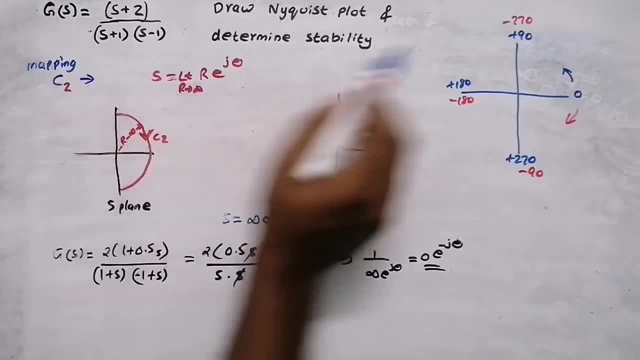 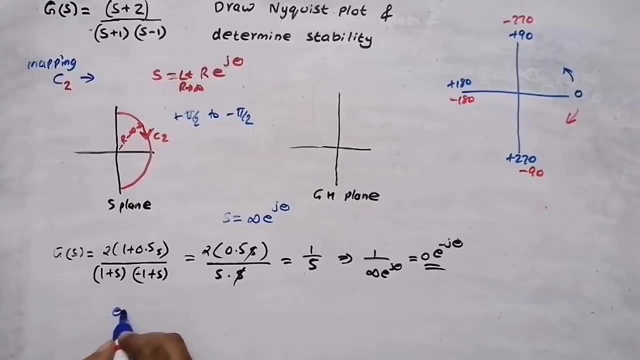 from the direction is like this: Okay, So theta is varying from plus 90 to minus 90. That is, plus pi by 2 to minus pi by 2. So when theta equal to pi by 2, we are going. 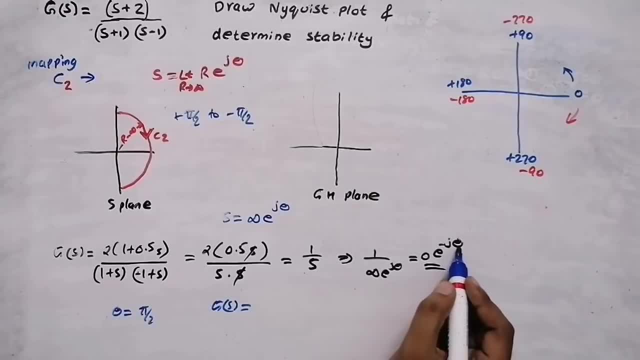 to find the corresponding g of s. Substitute theta equal to pi by 2 here. So we are going to get 0 e raised to minus j. Then for theta you need to substitute pi by 2.. It will become pi by 2.. Now, when theta equal to minus pi by 2, theta equal to minus pi by 2, my g of 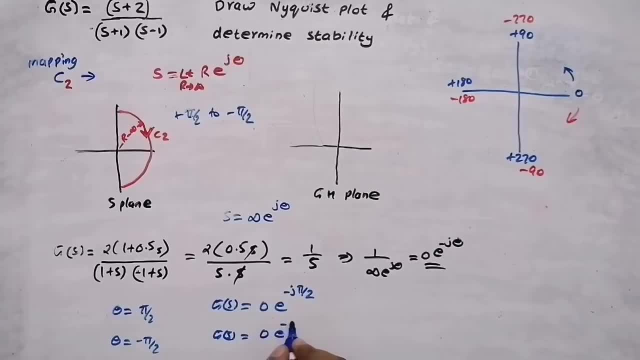 s will be magnitude equal to 0.. Then e raised to minus j Instead of theta right, minus pi by 2.. So minus and minus, it will get cancelled. We will get plus pi by 2.. Actually. 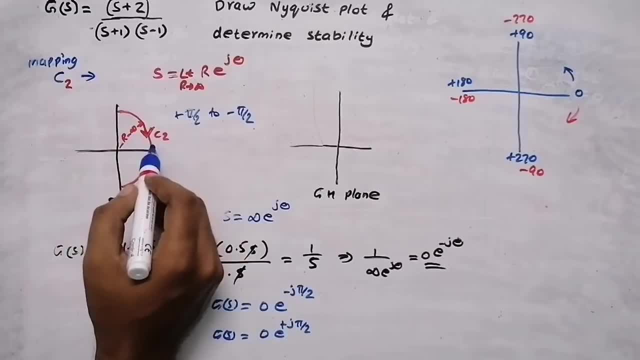 here theta is varying from plus pi by 2 to minus pi by 2 through 0.. Okay, Through 0, it is going Okay. Now we are going to map Okay From s plane if theta equal to plus. 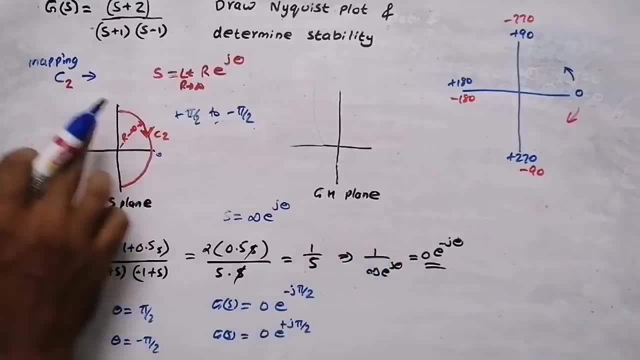 pi by 2, my corresponding g of s will be 0.. Okay, Now we are going to map. Okay From s plane. my corresponding point in g, h plane will be Here: when theta equal to plus pi by 2, here my g of s is 0 e raised to minus pi by 2.. Minus pi by 2 is minus 90.. So in 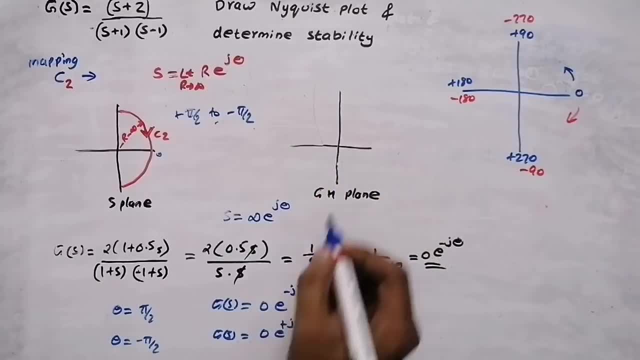 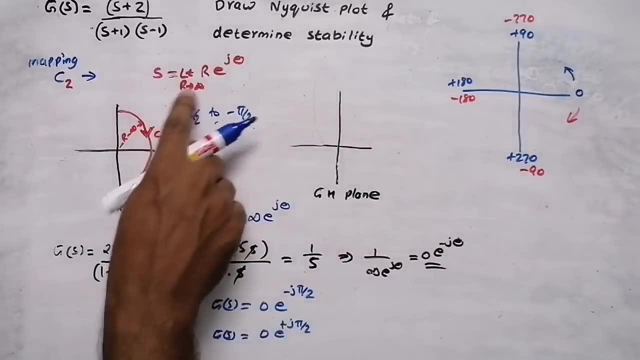 this axis. Okay, Magnitude is 0.. That means the point is going to be at the origin, But when you zoom it you can see a small circle. Here the radius is turning to 0.. Here the radius is turning to infinity. Here radius is turning to 0.. So we will draw a small 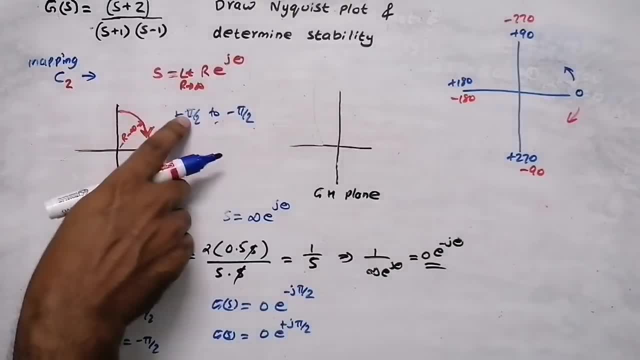 circle. Okay, Starting from here, starting from this point, that is plus pi by 2.. Here, when I substitute plus pi by 2, I am getting minus pi by 2.. So my point will be at this axis: minus 90.. 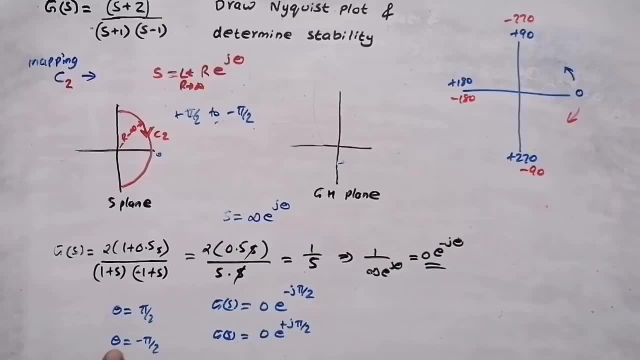 Minus pi by 2 at this axis. Okay, Now when theta equal to minus pi by 2, that means when I reach here- okay, through 0, I reached minus pi by 2.. The corresponding point in g, h plane is plus pi by 2.. So my plus pi by 2.. So my graph is going from minus pi. 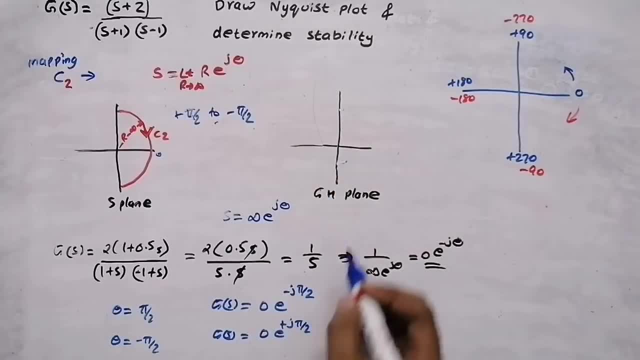 by 2, from minus pi by 2 to plus pi by 2.. So from minus pi by 2 through 0 to plus pi by 2.. Minus 90 to plus 90. So minus pi by 2 to plus 90. And my direction will be like: 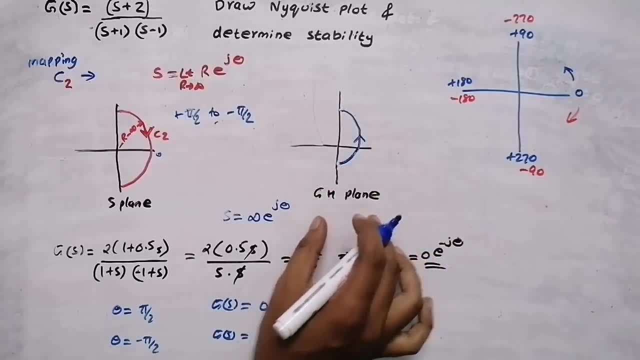 this: Okay. So this is the corresponding figure in g h plane. Here it is in s plane. The direction will be like this: Okay, So this is the corresponding figure in g h plane. Here it is in s plane. The direction will be like this: Okay, So this is the corresponding. 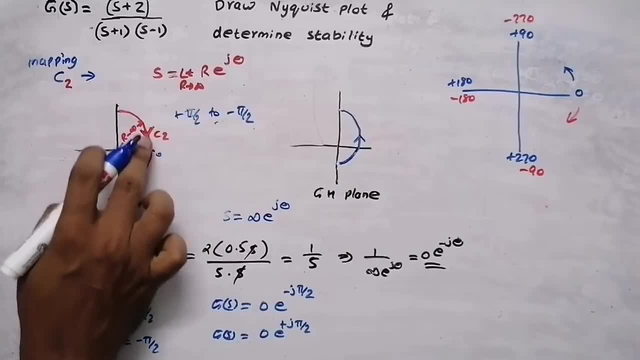 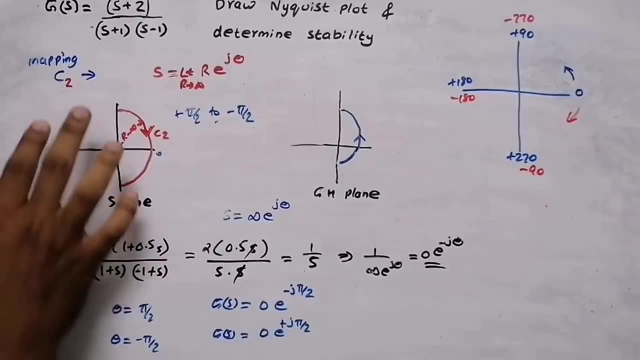 is from plus pi by 2 to minus pi by 2.. Plus pi by 2 to minus pi by 2.. In g h plane, minus pi by 2 to plus pi by 2.. Minus pi by 2 to plus pi by 2.. So for mapping region C2, write. 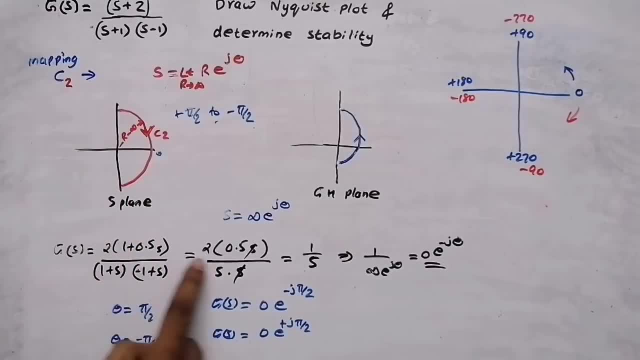 g of s, remove that 1 plus terms and write the remaining terms. Then, instead of s, you need to substitute r, e raised to j theta. But as you know, r is infinity, So we can write infinity e raised to j theta. So wherever there is s, replace it with infinity e raised. 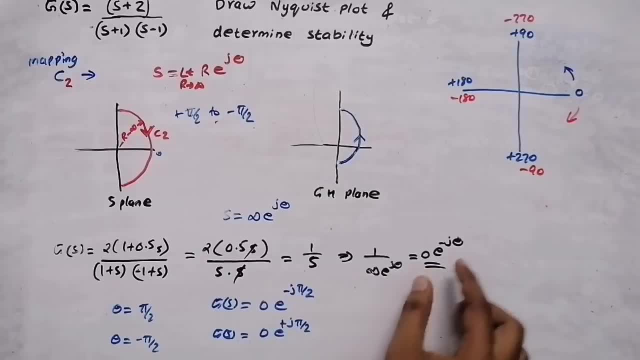 to j theta. So we will get the equation like this: 1 by infinity is 0.. So now for theta. here theta is varying from plus pi by 2 to plus pi by 2.. So we will get the equation. 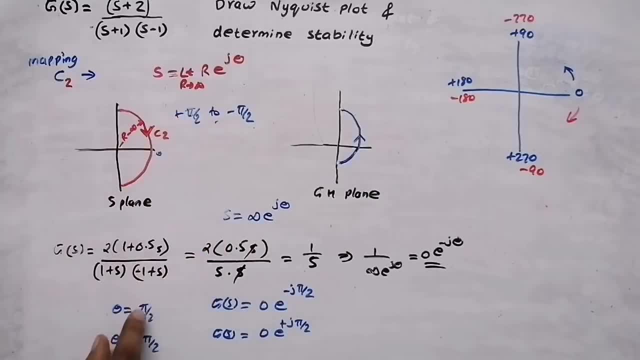 of minus pi by 2.. So first of all find: when we substitute theta equal to pi by 2, we will get g of s. Then when we substitute theta equal to minus pi by 2, we will get g of s. Using that, draw the plot in g h plane. Now we are going to plot our third region. 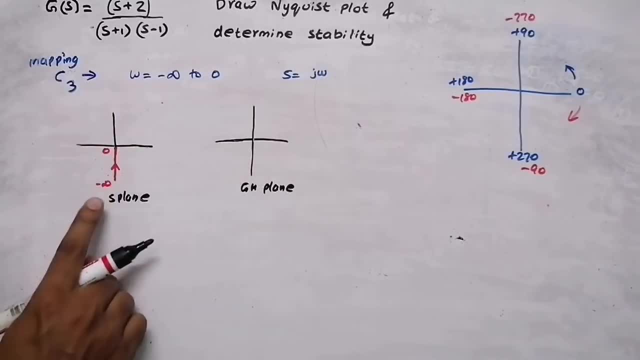 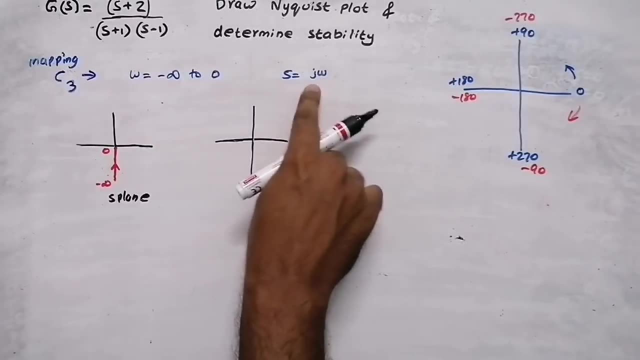 Third region is from omega equal to minus infinity to 0.. Minus infinity to 0.. This is in s plane. We need to find the corresponding figure in g h plane. At this point, what we will do? Instead of s, we will write j omega. We already found what is s equal to j omega. 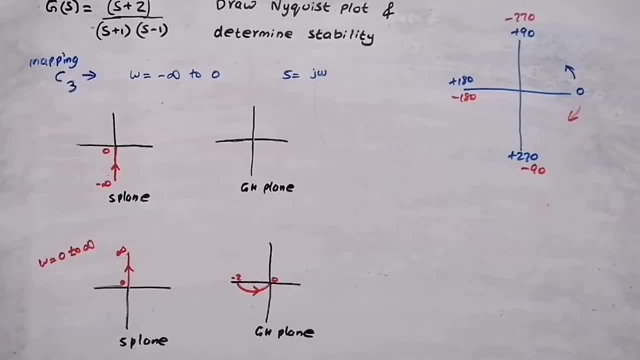 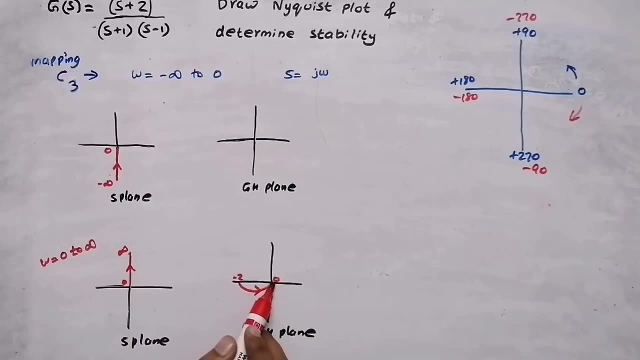 in the first region. So in the first region, that is, from omega equal to 0 to infinity, 0 to infinity. So we got the figure in g h plane like this, Starting from minus 2, the direction like this: up to 0. In this case it will be just the opposite- Okay, Just opposite- Here. if 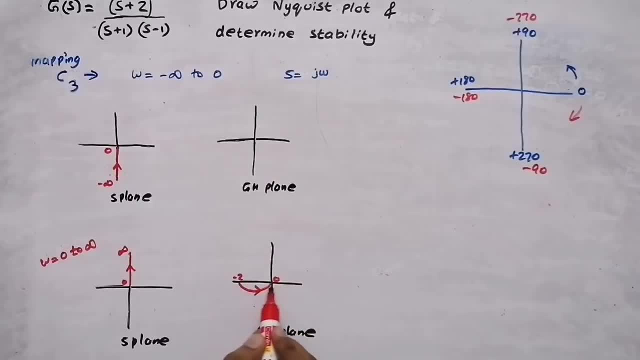 you are getting like this: then here from minus 2 to 0. Then here it will be 0 to minus 2.. Okay, From 0 to minus 2.. And here the direction is from minus 2 to 0. But here 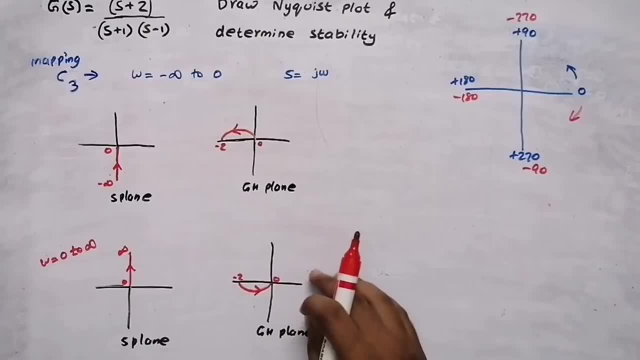 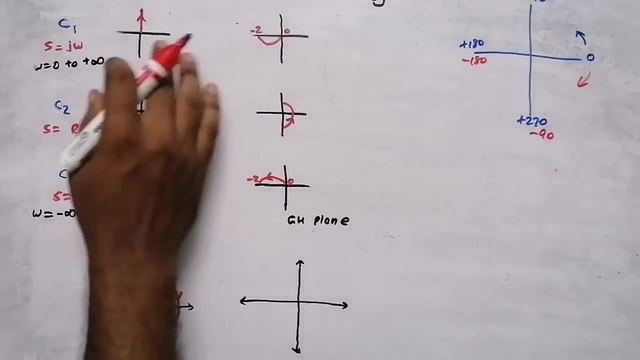 the direction is going to be 0 to minus 2.. So the inverse of this figure, or the mirror image of the first region, is our third region. So, after mapping, these are the regions that I get. I got this region. When I map c2, I got this region. When I map c3, I got this region. 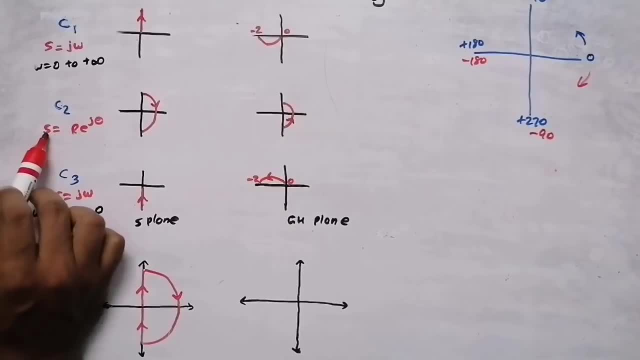 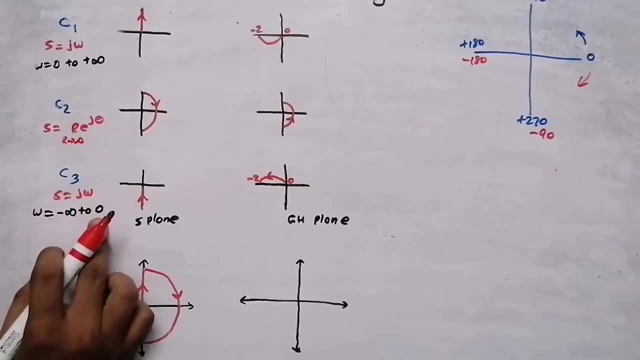 Okay, Here I substitute s equal to j omega. Here instead of s I write r. e raised to j theta, where r tends to infinity. Okay, And here I substitute s equal to j omega. Omega is varying from minus infinity to 0.. The corresponding figure in g h plane I obtained: 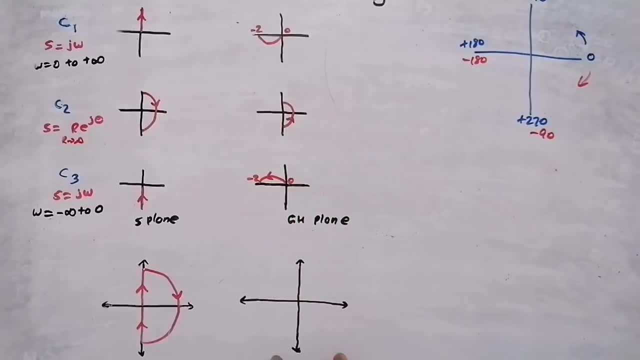 is this thing: Using this g h plane, we are going to draw the final plot. So the plot is going to start from minus 2.. Minus 2 to 0., So starting from minus 2.. Okay, Starting. 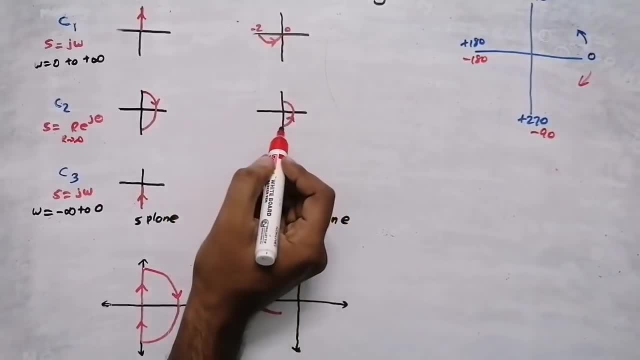 from minus 2, it is not going to 0.. It is going to 0.. It is going to 0.. It is going to this point. Okay, When I am going to combine this, it is not going to 0.. Instead of that, 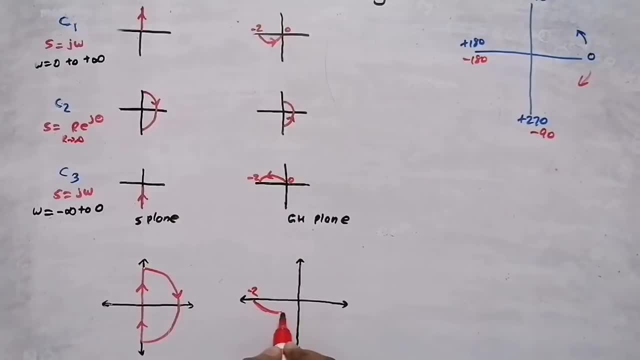 after reaching here, it will go to this point. So it will go to this point here. Now it will go like this: From minus pi by 2 to pi by 2.. So from minus pi by 2 to plus pi by. 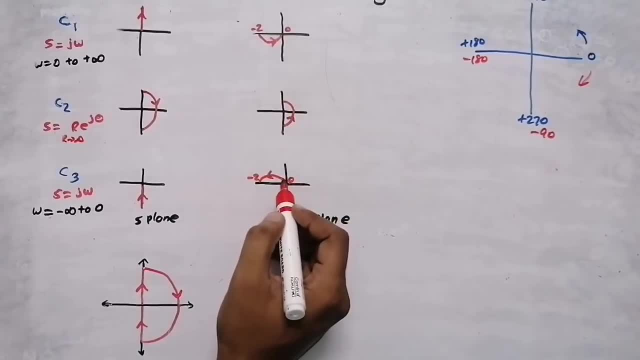 2, it will reach Then from here. instead of this, starting from 0,, it will start from like this: Okay, From 0 to minus 2.. So this will be my plot. So starting from minus 2. 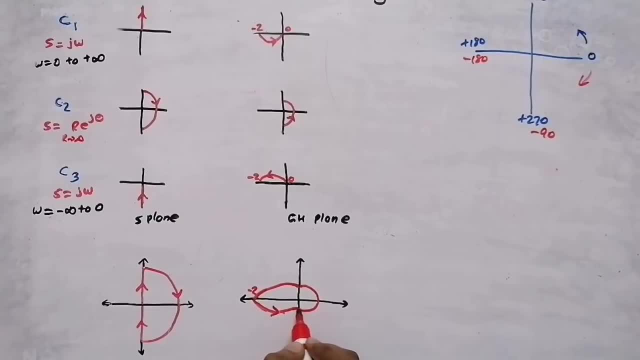 to 0. The direction will be like this Then: from here the angle will be minus pi by 2 to plus pi by 2.. We already found that. Okay, So the direction will be like this Then. actually. 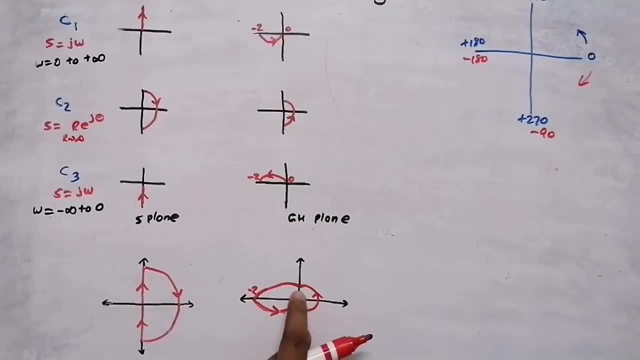 this plot is starting from 0.. But combining after combining, we will get like this: It will not start from 0.. Instead of that, it will be a continuation of this graph, So starting from here like this. So this will be our final Nyquist plot, After drawing the 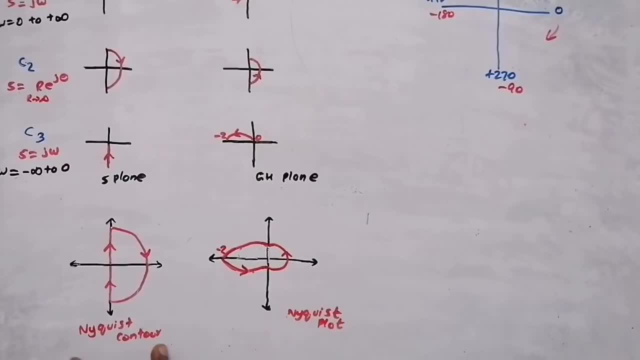 Nyquist plot we need to find the stability. In S plane we will find stability with respect to origin, But in Nyquist plot we will find stability with respect to the point minus 1 plus j0. Here imaginary time is 0.. Okay, With respect to this point we will tend the stability. 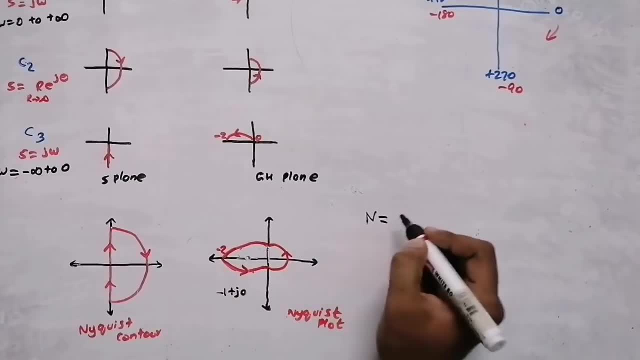 Now how to find stability. As we know, n equal to P minus Z. This is the equation used to find the stability. Now, what is n, What is p and what is Z? n is the number of encirclement across this. 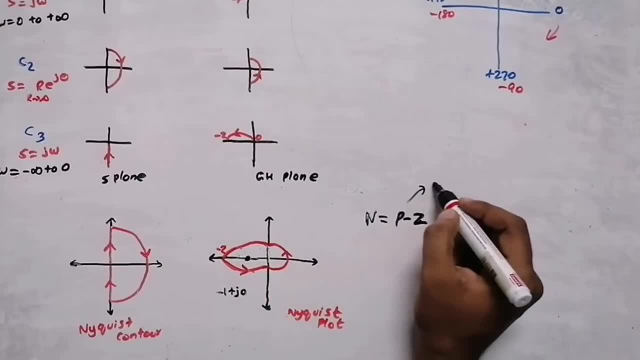 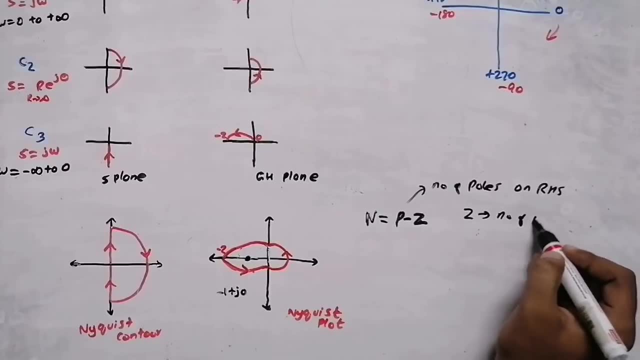 point. Okay, P is the number of poles. number of poles on arches on the right hand side. Z is the number of poles on arches. Oh, Yes, Okay. Here is the number of arches. The number issues this part. This is just Ad체적ura. Because of that, since the imagem is Bret kriege, we think it is none other than 0.. Because here i amφ and mx and vs were applied. the meineigkeit: 741285. 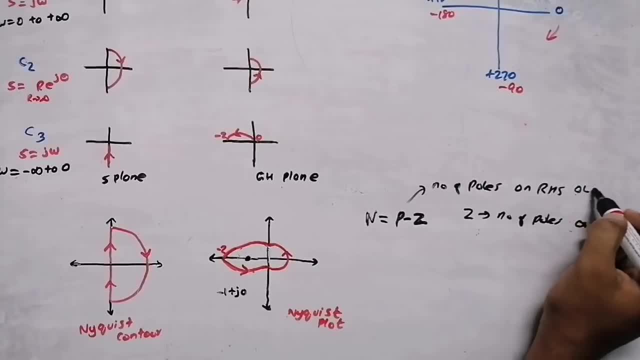 so here the number of poles is for open-loop system. okay, here it is for closed-loop system. this is the number of poles of closed-loop system. here the number is number of poles of open-loop system. so at the end of the equation we need to find the value of z. from this we will get z. 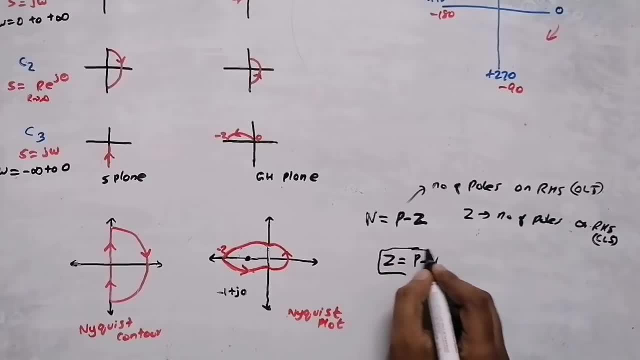 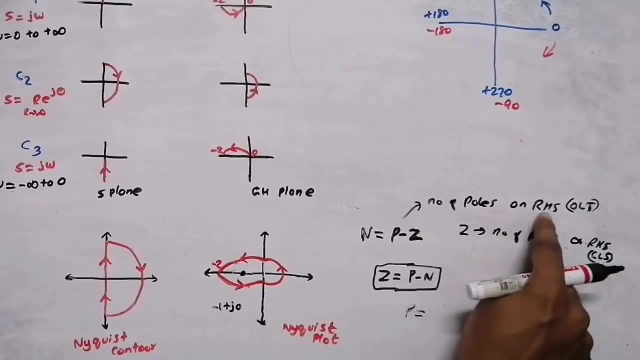 equal to p minus n. this is the equation used to find the stability. okay, now, first of all, we can find the p. okay, p value. what is p? number of poles on arches of open-loop system. so this is our open loop system for finding the poles. we will equal denominator equal to zero. at that time we will. 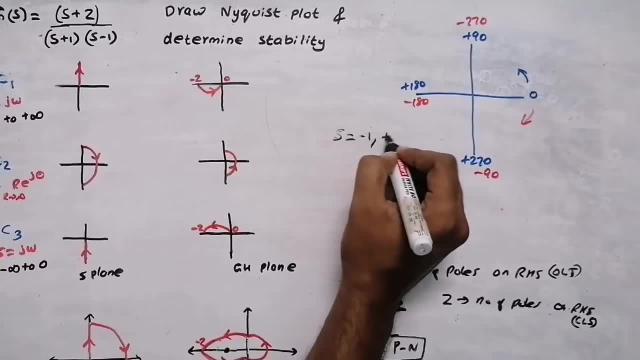 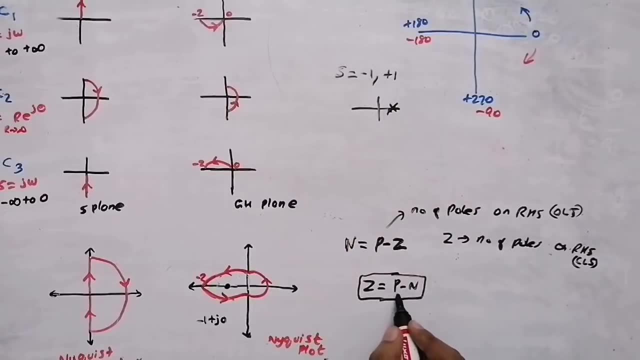 get either s equal to minus one or we will get s equal to plus one. plus one means there is a pole on the right hand side. so when there is a pole on the right hand side, we will get p equal to one. there is one pole on the right hand side, now minus n. how to find n? n is the number of encirclement. 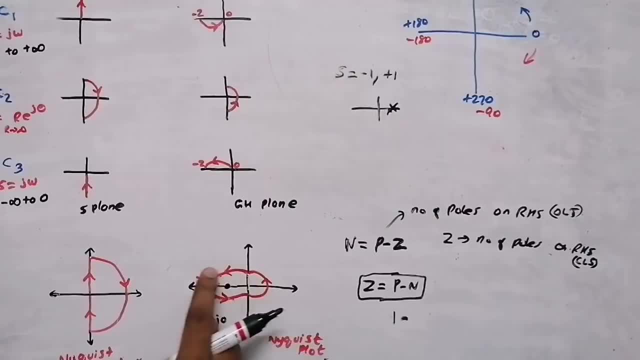 around this point. if encirclement is in anti-cropwise direction, n is positive. so here there is only one encirclement around this point, so it will be one. if there are two encirclement in anti-cropwise direction, it will become two. n will be positive. 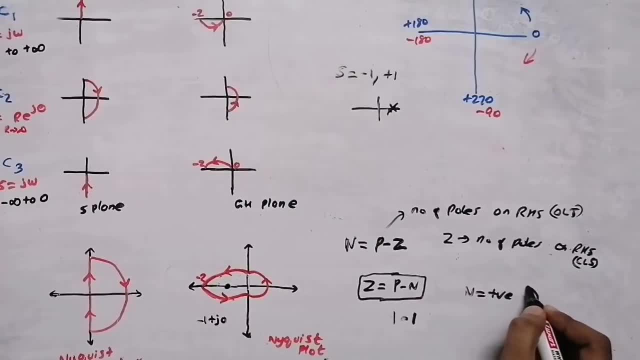 n is positive when encirclement is in anti-cropwise direction. actually n is positive. but because of this minus a, here this minus come okay, here there is a minus a. because of that, this minus a, actually n is positive. there is only one encirclement, so the value of n it is one. 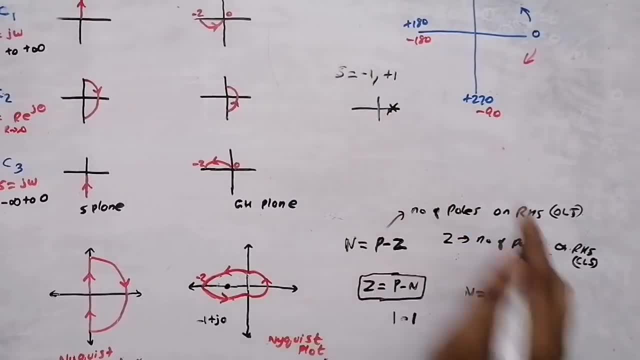 the value of p also one. there is one pole on the right hand side, so p is one, n is one. you will get one minus one. it is zero. so z equal to zero. that means number of poles on right hand side of closed-loop system is zero.